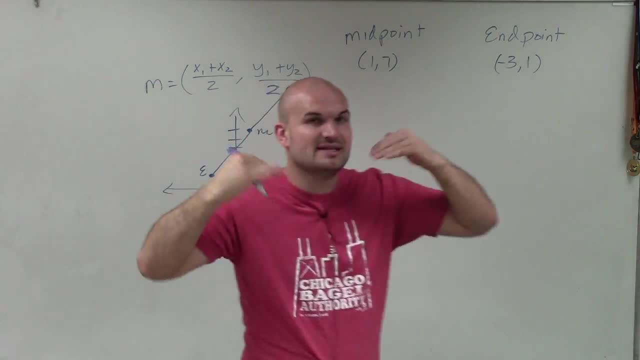 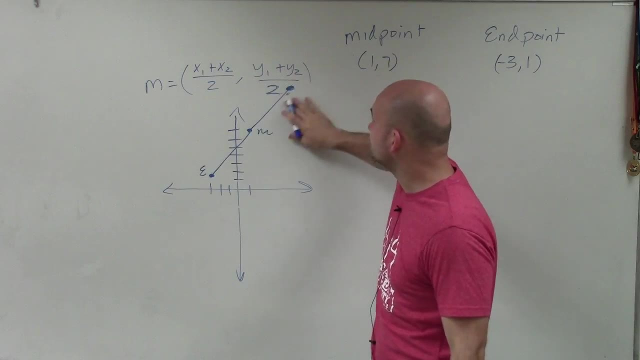 but we need to figure out what this point is. So, going with the understanding of what a midpoint is, it's directly in between your two endpoints. The problem is, we just don't know this endpoint. Now, what I can do is say: so, this endpoint. 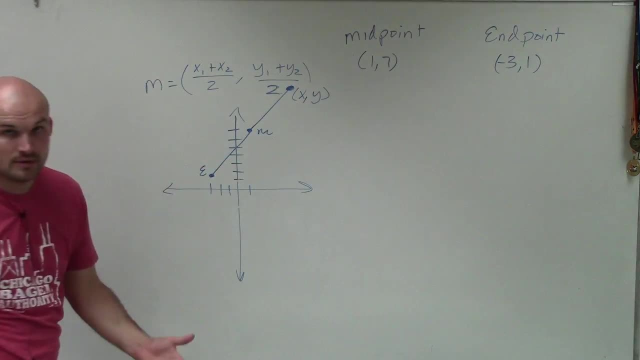 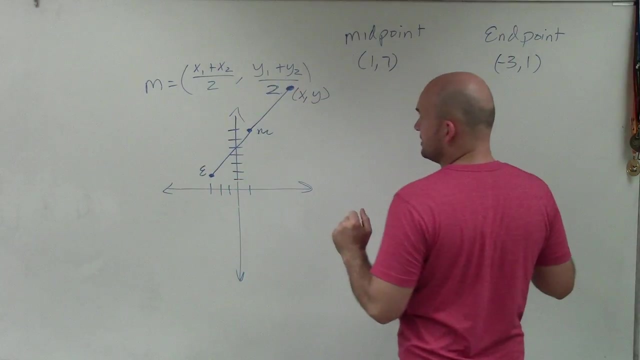 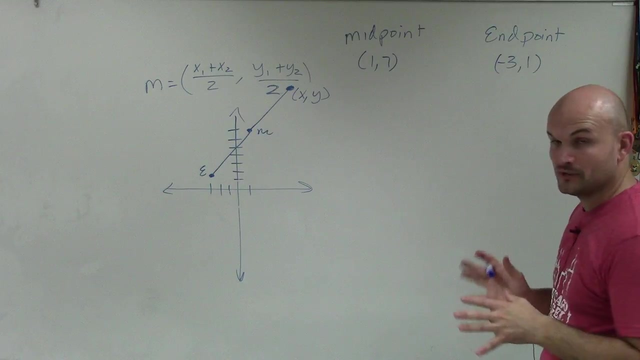 is going to be some x and y-coordinate which we do not know right. So the only thing we can say is what we're going to do is we know the midpoint, but we do not know what the x and the y value is for the endpoint. 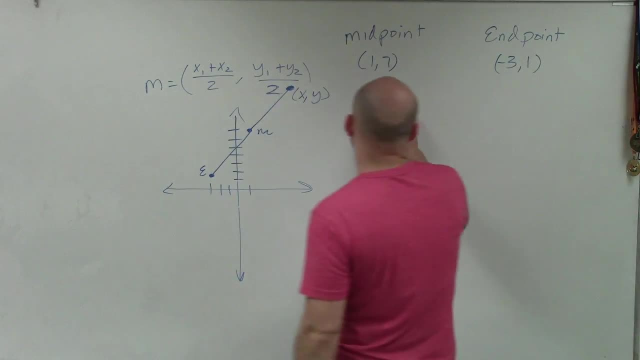 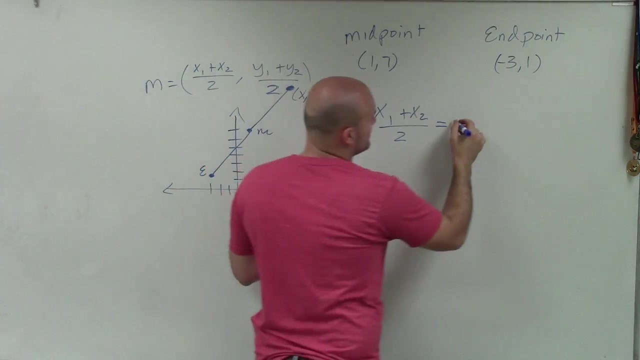 So what I'm going to do is I'm going to take my midpoint formula and I'm going to break it up. So I'm going to say: x1 plus x2 divided by 2, equals. remember that- equals the midpoint, the x3. 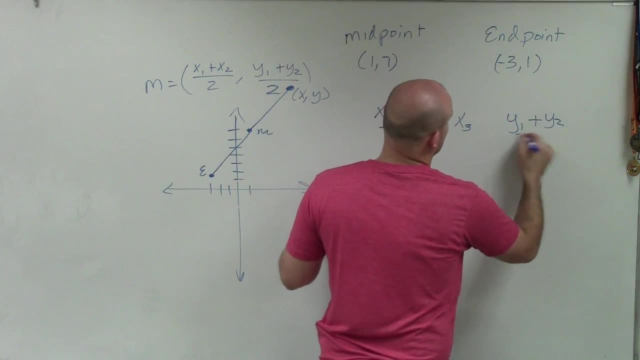 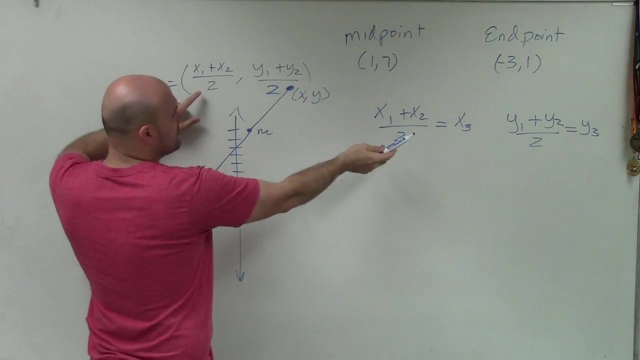 And let's do y1 plus y2.. y2 divided by 2 equals y3, right Now, what was y3?? What was x1 and x3 and y3?? x3 and y3 is what happened when we got these values right. 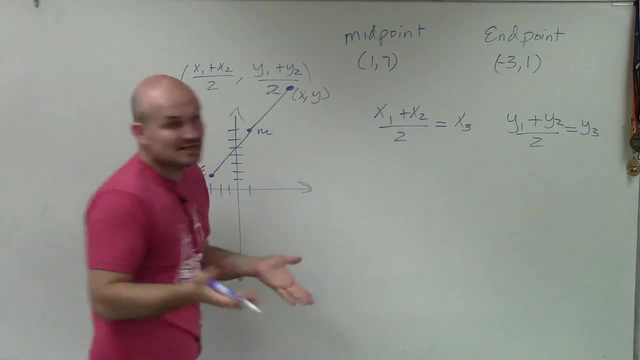 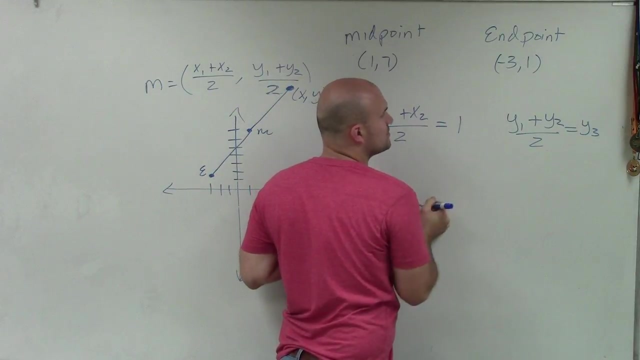 Which are the values of the midpoint. So do we know the values of the midpoint? Yes, we know that x value of the midpoint is 1.. So instead of using x3, I'm going to say the midpoint was 1.. The y-coordinate of the midpoint was 7.. 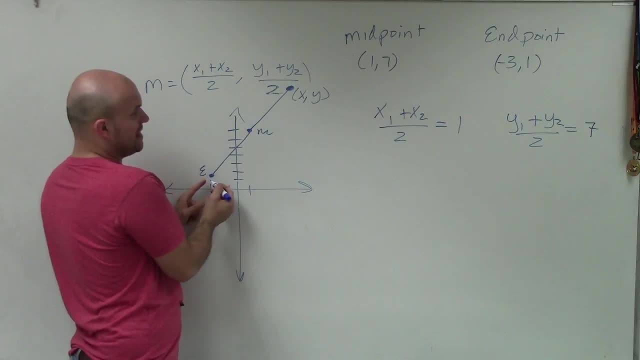 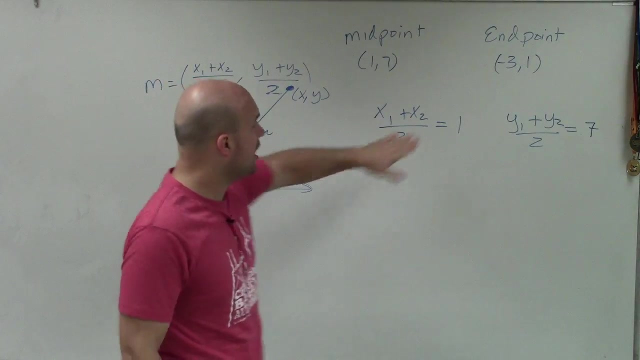 Now Of the endpoints. we know one value of the endpoint, But we don't know the other x. right, We know one x, but we don't know the other x. So what we're going to do is we're going to plug in our endpoints in 1 for x and 1 for y. 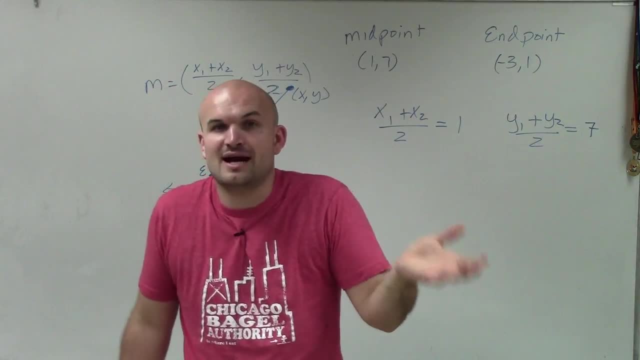 Now determine if it should be for x1 or y1, or x1 or x2, y1 or y2.. It doesn't really matter, You just need to choose. So let's plug them in for x1 and y1. 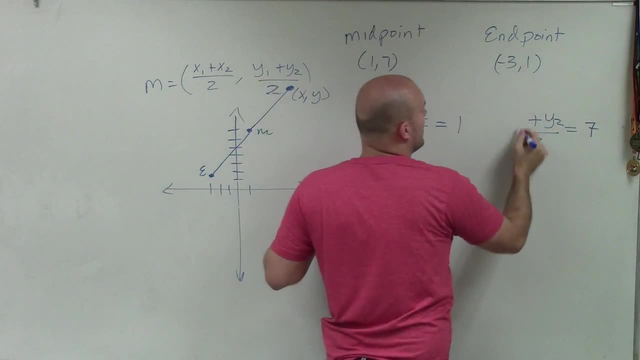 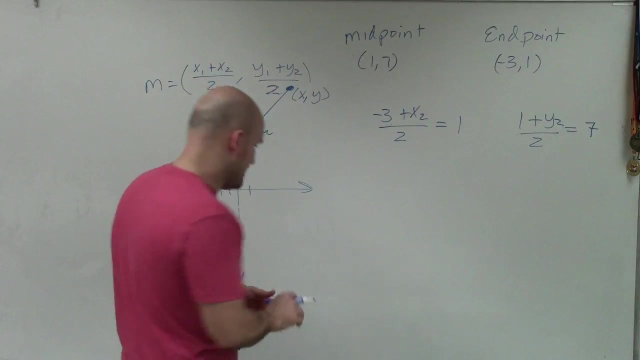 So x1 is going to be my first point in my endpoint, which is negative 3.. And y1,, which would be 1.. Now you can see, I have an equation that I can go ahead and solve for x. So to do that, I need to apply my inverse operations. 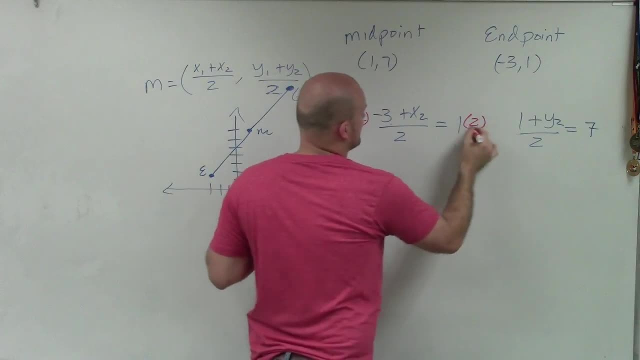 So I need to get the 2 off the bottom. So I'll multiply by 2 on both sides. These 2's divide to 1. And therefore I'm left with a negative. 3 plus x2 equals 2.. Now I use my inverse operations again.